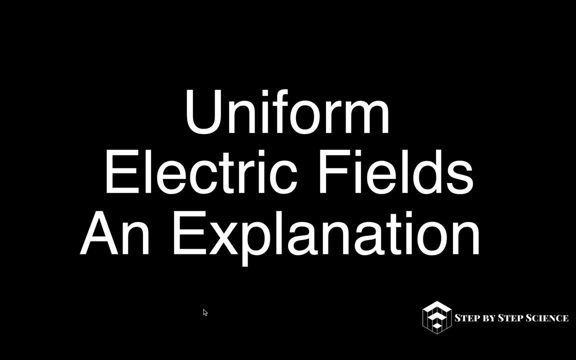 In today's video we're going to go over an explanation of uniform electric fields, and that is? uniform electric fields are fields that exist between charge parallel plates. Now, before you get started, please don't forget to subscribe to my channel, Step-by-Step Science. 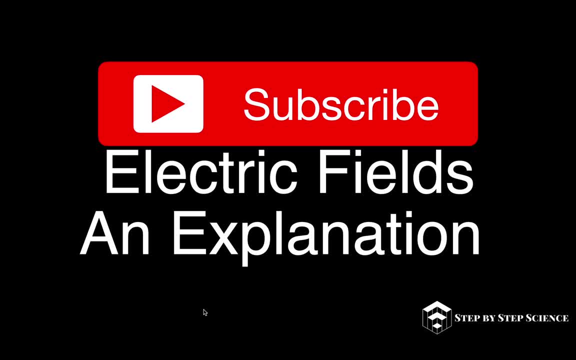 Get all of our amazing physics, chemistry and math videos. Please subscribe, click the notifications bell, give us a thumbs up, leave us a positive comment and don't forget to share this video. And in addition to that, I've made a bunch of other teaching and learning material. 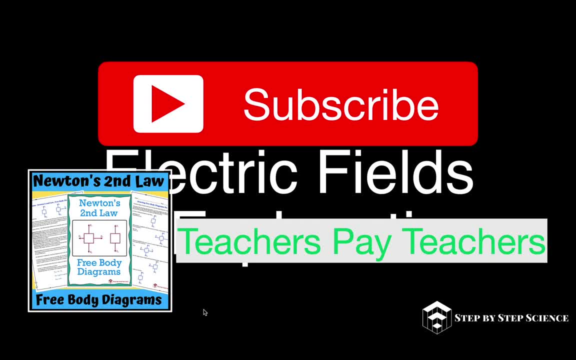 that you can find on my Teachers Pay Teachers website, Whether you're looking for practice problems, notes, example, problems with all the solutions, some puzzles that you can work on and also some great activities that you can do with PGT Interactive Simulations. 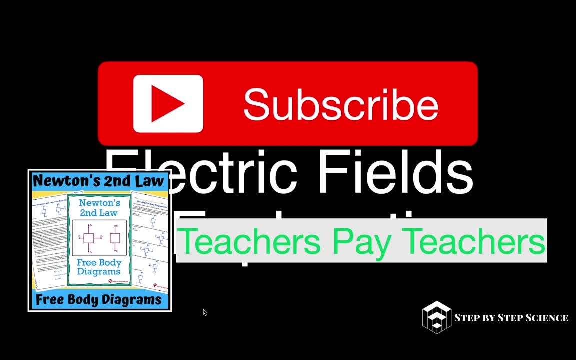 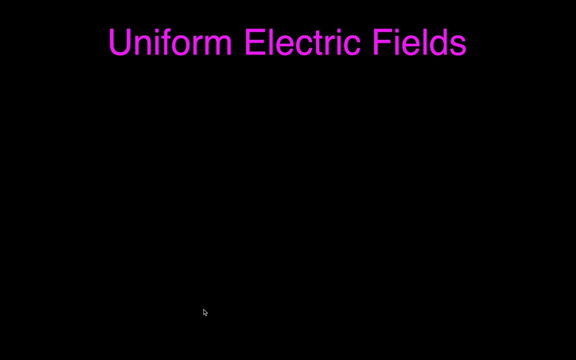 it's all available at my Teachers Pay Teachers website. The link is in the description below and let's go. This is uniform electric fields, and uniform electric fields, as I said, are fields that exist between charged parallel plates And when we have charged parallel plates. 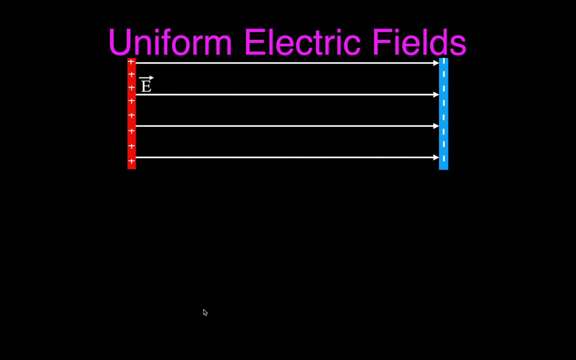 between those plates we're going to have an electric field, and the electric field is going to be the electric field that we're going to be using. And when we have charged parallel plates, we're going to have an electric field, and the electric field always goes from the positive to the negative plate. All right, 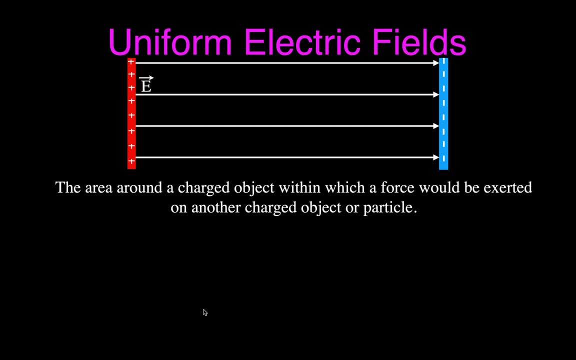 now, what's kind of a definition? a nice good definition for electric fields. This works for either uniform fields or non-uniform fields. It's the area around a charged object in which a force would be exerted upon another charged object or particle. All right, and also we have uniform. 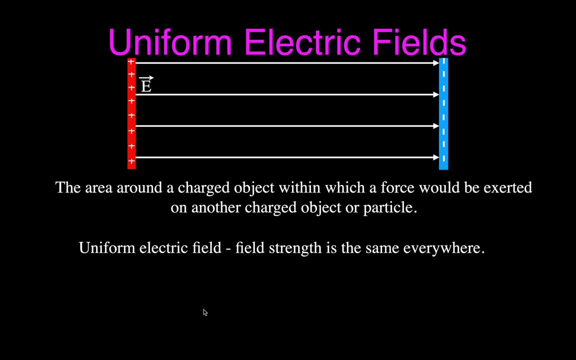 electric fields. Then we say that the field strength is everywhere the same. So between those charged plates we have an electric field and we say that the field strength is everywhere. you see three shades of blue. Well, it kind of fits the picture. That's the alphabets. 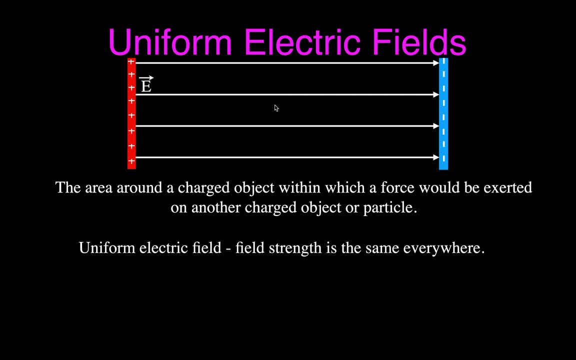 So you can see the field lines are equally spaced and that shows as diagrammatically, that's kind of an indication that the uniform field, the field between those plates, is uniform. Also, as we said, the field lines always flow from the positive plate to the negative plate. 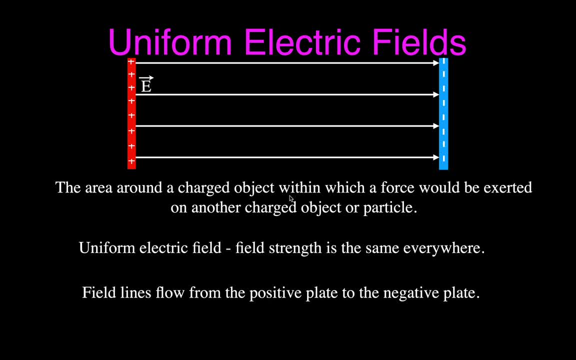 Okay, now up here we said it's the area in which a force would be exerted on another charged particle. so if I put a positively charged particle in that electric field, it's going to feel a force to the right from the electric field and that's kind of that direction. 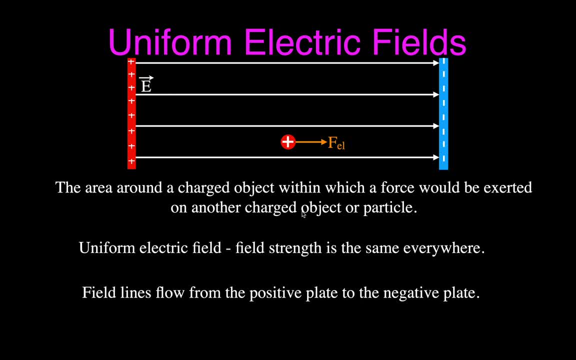 That's how we define the direction of the electric field. It's the direction of the force on a positively charged particle. Obviously, if we put a negatively charged particle, then it's going to feel a force in the opposite direction. All right, so this is kind of a description of the 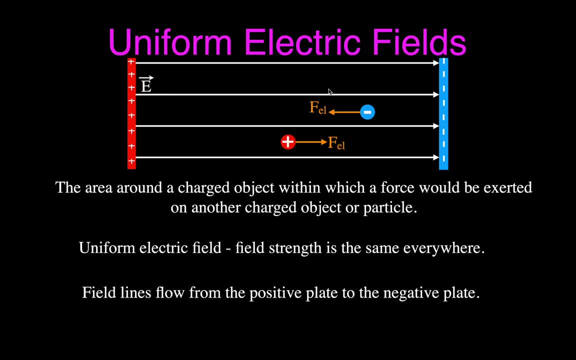 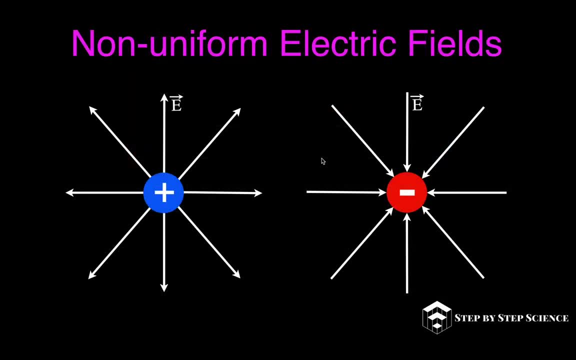 electric field and it's uniform. and you can see that it's uniform because the field lines are equally spaced. That is different than if we have a non-uniform field around a charged particle, a point charge, and you can see these are non-uniform electric fields because the closer you are to the 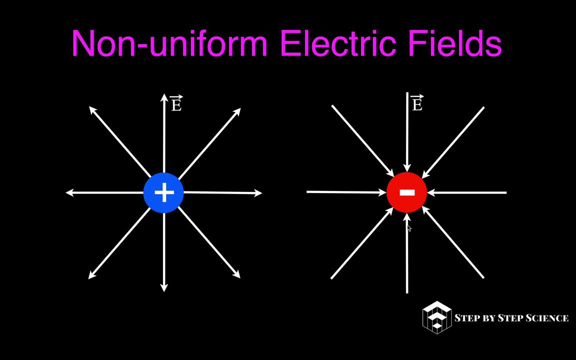 charged particle, the closer the lines are together, and that's an indication that the field strength is stronger closer to the particle and the farther away you get, the greater the spacing is between the electric field lines, and that's an indication that as you move away from each of 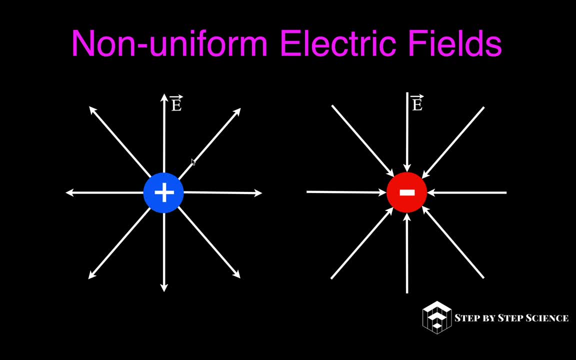 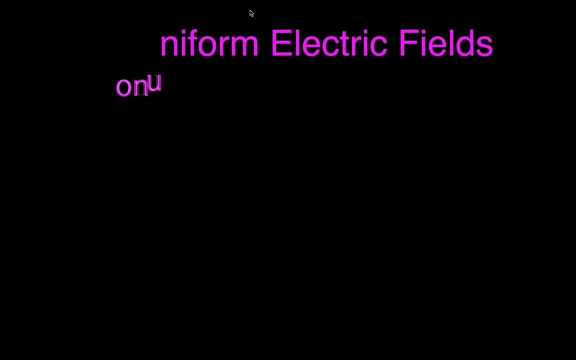 those charged particles That the field strength decreases as you move away. You can still see that the field lines go from a positive charge to a negative charge. but these are non-uniform electric fields that we see around a point charge. Okay, just as a comparison for uniform field. Now back to our uniform fields. 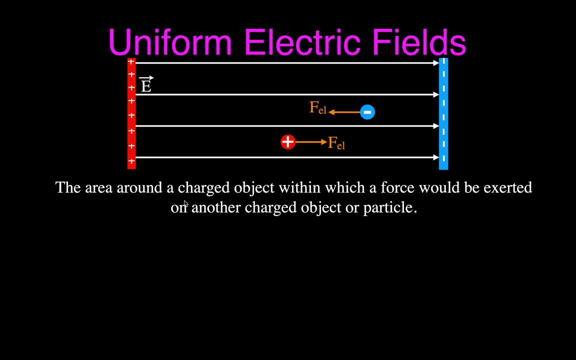 we had our description here. Now, mathematically we define the electric field. it's defined as the force on a tiny positive test charge. I always say a tiny positive test charge. It's a force on a tiny positive test charge. It's a force on a tiny positive test charge. 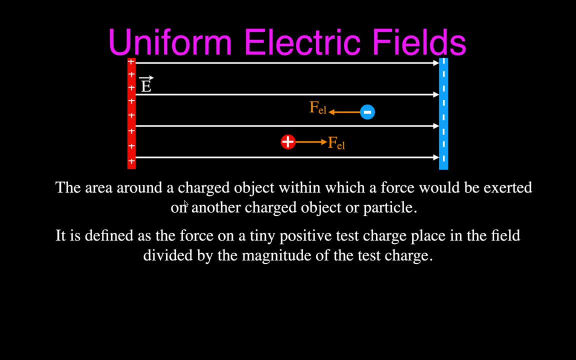 That's not going to disrupt the field. I just think of it as the force on a test charge, on a positive charge, that's placed in the field, divided by the magnitude of that charge or that test charge, and we would write that out mathematically in an equation. The symbol for the electric field is E. 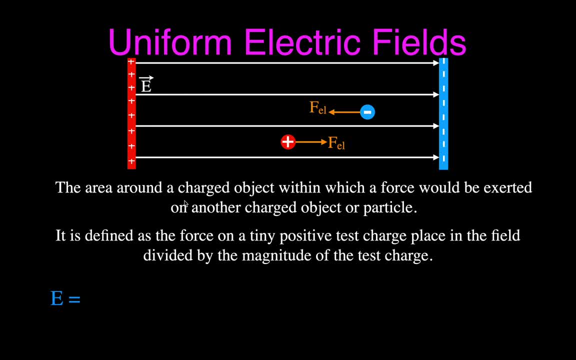 It's a vector quantity and, as you can see by the definition here, it's just the force divided by the charge. so we write down the force divided by the charge. The force will be measured in newtons. The charge will be measured in coulombs. 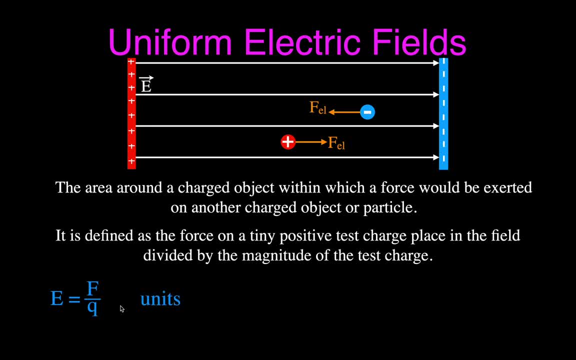 So when we use this equation to calculate the electric field strength, the units are going to be in newtons per coulomb, like that. Now there's another equation, another set of units that we can use to define the electric field. They're equivalent with the newtons per coulomb, and that's. 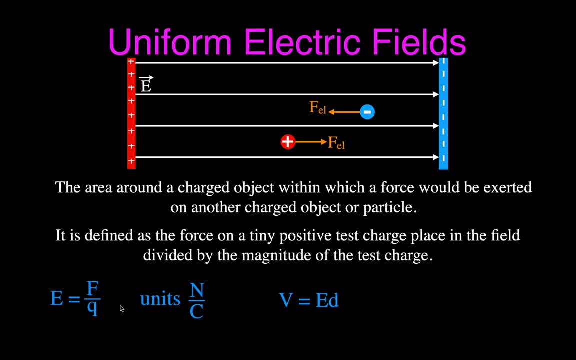 when you have this equation, which also has the electric field, and we can use this equation for parallel plates, not for point charges, but this equation is used for parallel plates. It says that the voltage, the potential difference between those two plates, is equal to the electric. 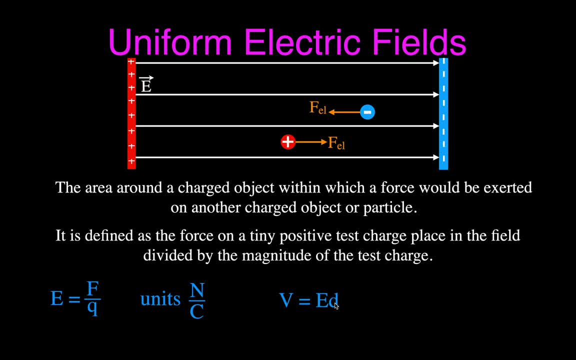 field strength times the distance between the plates. If we rearrange this equation and solve it for E, then we get the voltage divided by the distance and the voltage is measured, or the potential difference is measured in volts, The distance is measured in meters. so you see, we have. 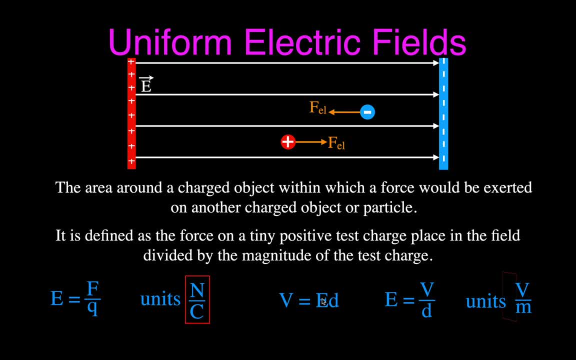 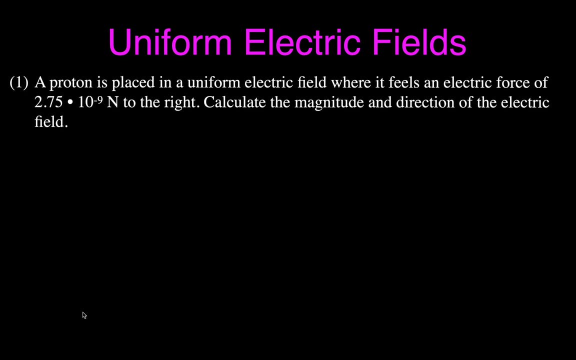 two equivalent units that we can use for the electric field strength, either newtons per coulomb or volts per meter. Either one works, depending on which equation that you're going to use. okay, Okay, Now let's go on and do some example problems. We have a proton. It says it's placed in a uniform. 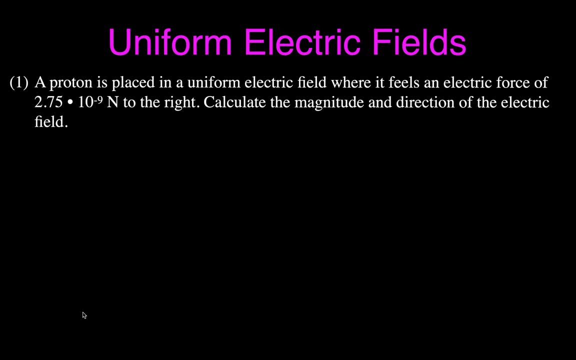 electric field where it feels an electric force, from the field of 2.75 times 10 to the minus newtons to the right, and we want to calculate the magnitude and the direction of the electric field. All right, so we have our positively charged particle and it's a proton and it has the force. 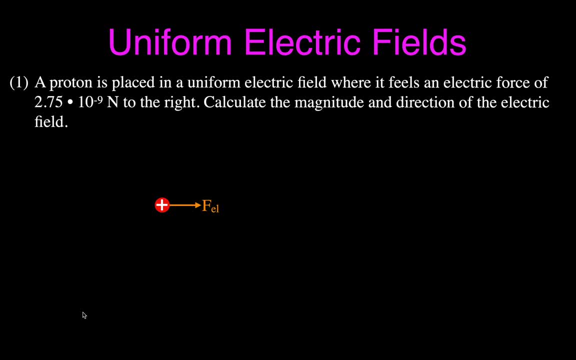 to the right, and we want to know the direction, the magnitude of the field. Well, if the force on a positively charged particle is to the right, then that means the field is also to the right, and then we could set up our parallel plates like: 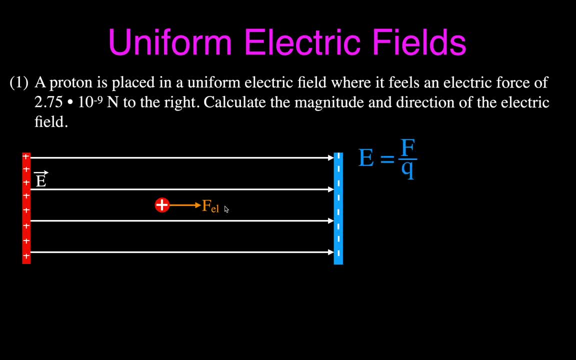 that The field goes from the positive to the negative. Now we just want to calculate the electric field strength. It's the force divided by the charge. We're given the force 2.75 times 10 to the minus 9 newtons. This is a proton, and you might know that the charge on a proton is 1.60. 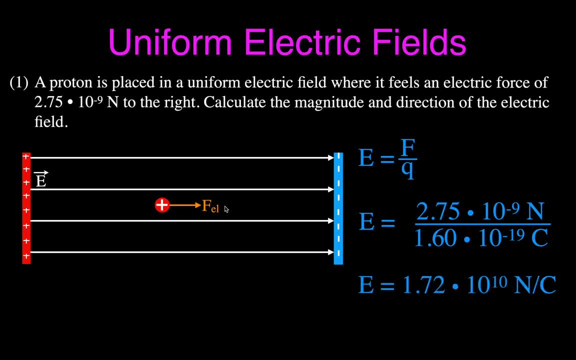 times 10 to the minus 19 coulombs. Divide those and you get that the electric field strength E is 1.72. Times 10 to the 10 newtons per coulomb. You can see. we're dividing newtons and coulombs, so we have the 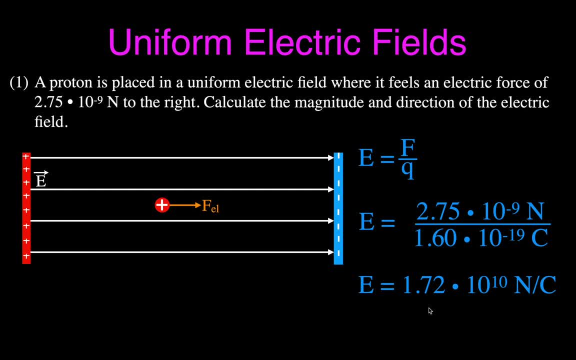 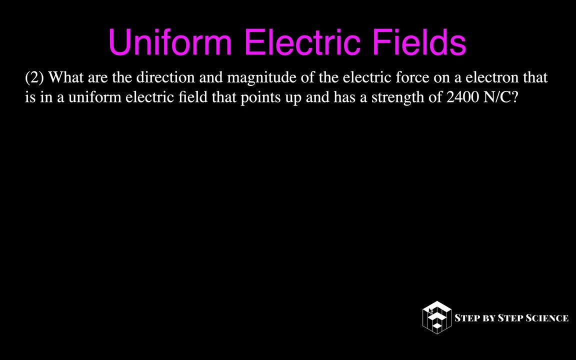 electric field strength in newtons per coulomb. That's number one and the field is to the right. Okay, number two says: here we have. we want to know now this case. we want to know what's the direction, the magnitude of the force on an electron, that is, in a uniform electric field. 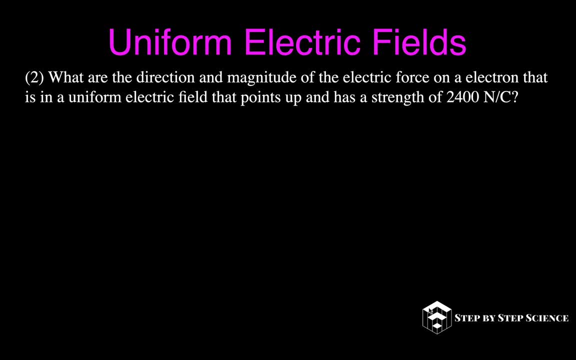 The force points up and the force strength is 2,400, 2,400 newtons per coulomb. We know that it points up in that direction And that means if we put our plates like that, we put an electron in there, that the force is going to be. 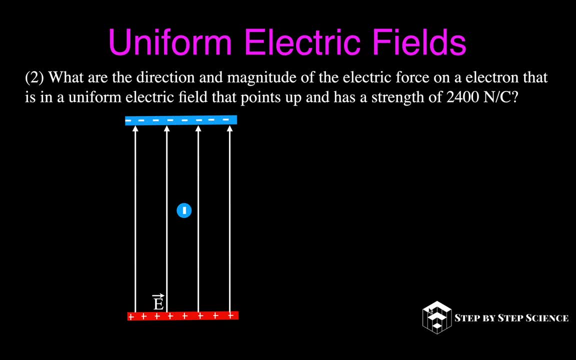 not in the opposite direction, of course, but it's going to be in the direction pointing downwards, as that charge is attracted to that positively charged plate and the force is in the opposite direction of the field and we want to know what is the amount of force. We're going to use this equation. 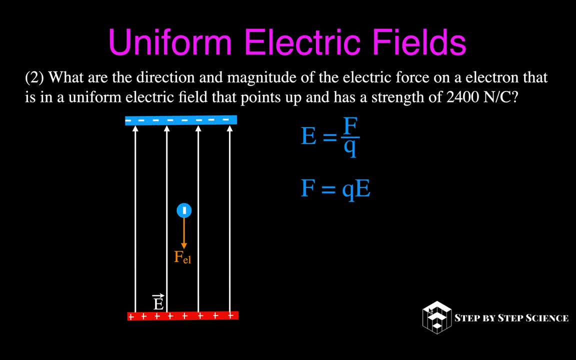 which we're going to solve for the force. It's just Q times E, It's an electron. you know, or you can look up, The charge on an electron is 1.60 times 10 to the minus 19.. Remember protons and 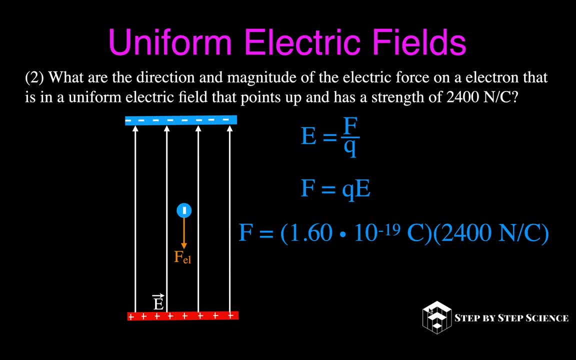 neutrons have the same charge, both in coulombs of course, and the electric field strength is 2400 newtons per coulomb. You can see that the coulombs are going to cancel and the force on that electron would be 3.84 times 10 to the minus 16 newtons. All right, and that would be in this. 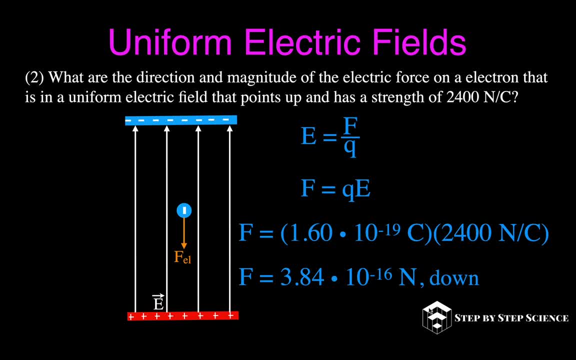 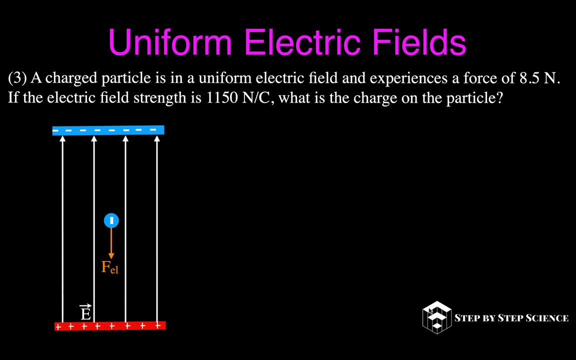 case, the way the field is oriented, the force would be in the downward direction. All right. number three is: it says a charged particle in a uniform electric field experiences a force of 8.5 newtons. If the field strength is 1150 newtons per coulomb, what is the charge? We used the same. 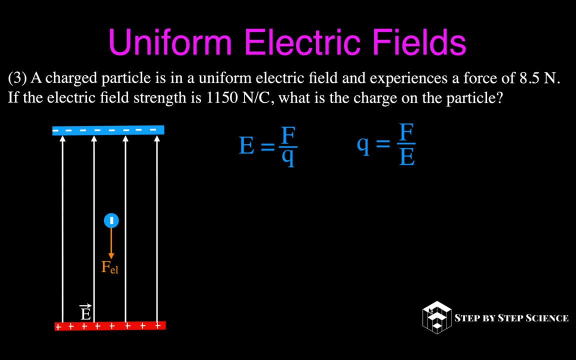 equation. Now we're just going to solve for the charge. It is the force divided by the field strength. We are given the force, It's 8.5 newtons, We're given the field strength and that means the charge of that negatively charged particle. 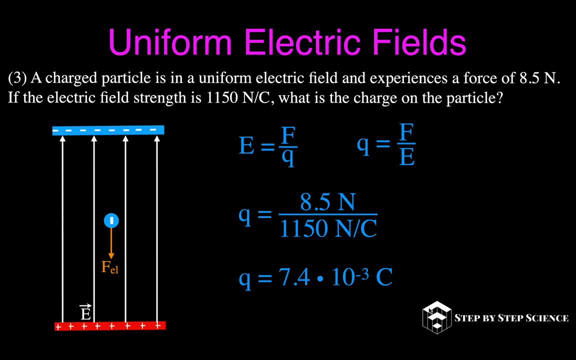 would be 7.4 times 10 to the minus 3 coulombs, or 7.4 millicoulombs like that. Okay, all right. Now for the other equation. it says here that there's a potential difference between the plates and the. 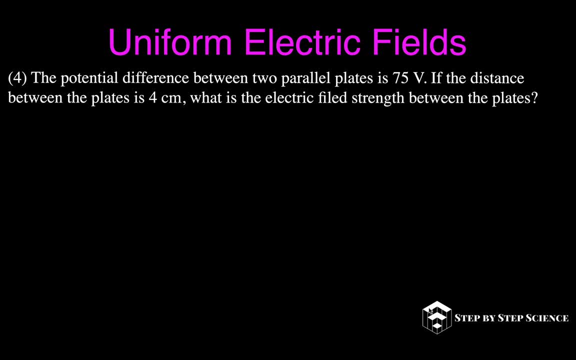 potential difference is 75 volts, The distance between the plates is 4 centimeters and we want to know what the electric field is. So we have the electric field strength is, we have our parallel plates, we have the electric field like that and we know that the difference between those two 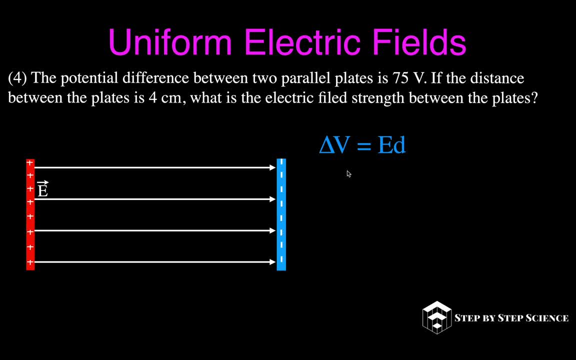 plates is 75. volts and we're going to use this equation because this has the volts in the distance and that's what we're given. We're going to rearrange to solve for the field strength. This is a change in the voltage. 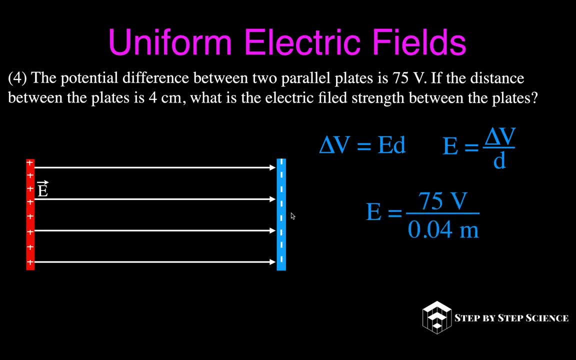 divided by the distance, and that would be 75 divided by 0.04.. Remember, you've got to convert, always two meters, and that means the electric field strength is 1875 volts per meter. All right, that's the electric field strength. We're using that equation. Okay, I think we have. 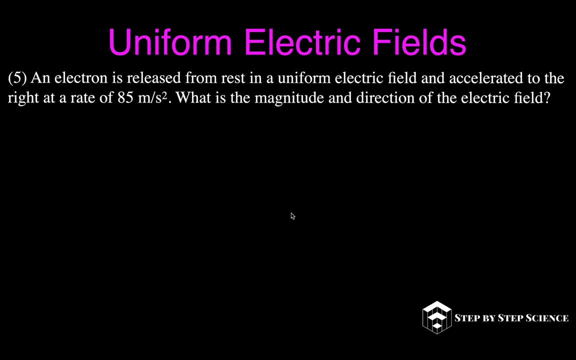 one more. All right, this is a little bit of a challenge question. We have an electron, It's released from rest in the uniform electric field. It has a certain acceleration of 885 meters per second and we want to know what is the magnitude and the direction of the electric field. All right, 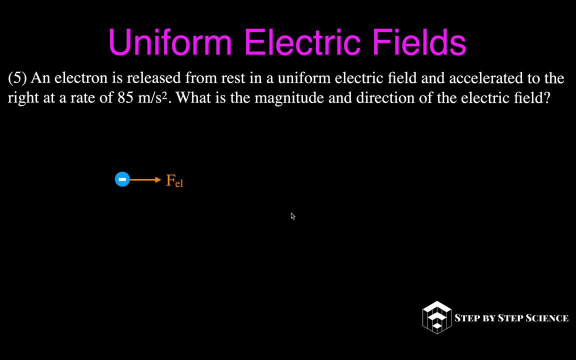 so we have our negatively charged particle. It's going to feel the force to the right and that means the field is in the opposite direction, to the left. Okay, that's the direction of the field. We can just draw our positive and negative plate in there like that. 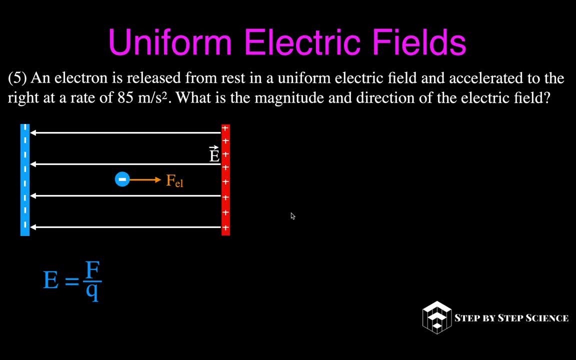 and we're going to use this equation to figure out the field strength, the force divided by the charge. except we don't know the force. but we can use Newton's second law- F equals ma- because we know the mass of an electron, We know the acceleration, and the mass of an electron is 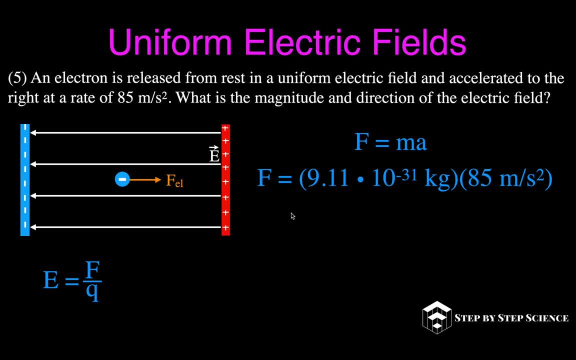 9.11 times 10 to the minus 31 kilograms. The acceleration, as it tells us, is 85 meters per second squared, so that electron is going to feel a force that would give it that acceleration would be 7.74 times 10 to the minus 29 newtons, and we can plug those values in along with the. 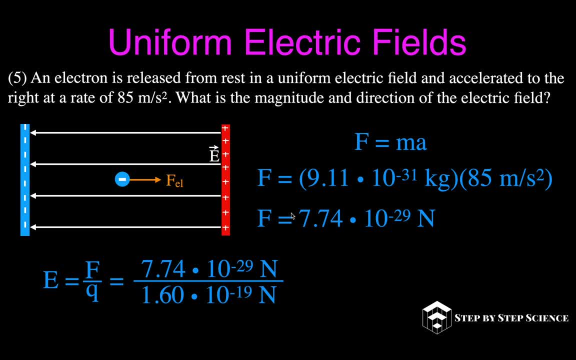 charge which we know for an electron is 1.6 times 10 to the minus 19 newtons, and that means that the field strength resulting from that acceleration of that electron is 4.84 times 10 to the minus 10. 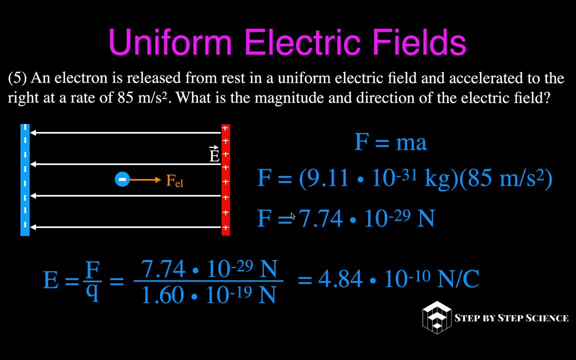 newtons per coulomb. Okay, so there you go. That's a quick overview, a quick explanation of what the electric field is for. uniform electric field, All right, it's the region where another charged particle will feel a force inside that field, and therefore we had those five excellent. 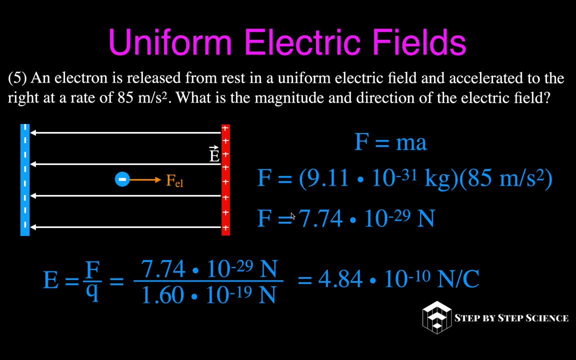 examples that we did. Okay, so thank you so much for watching. I hope you enjoyed the video. If you did, please don't forget, as I said before, to do the following five things. Please support our channel, Step-by-Step Science. Get all our excellent physics, chemistry and math videos. You should